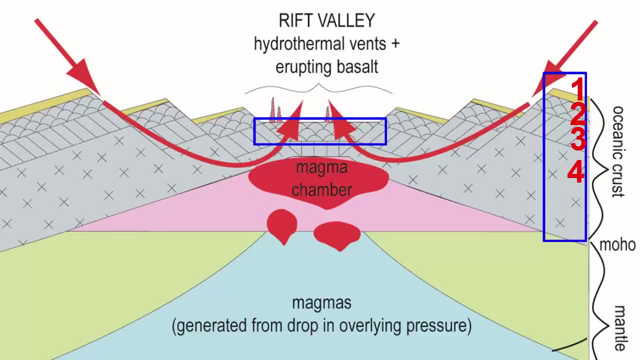 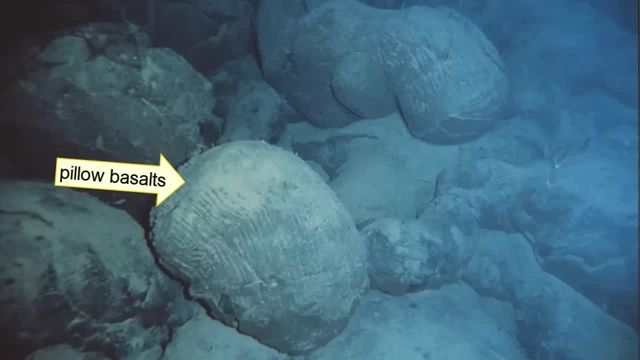 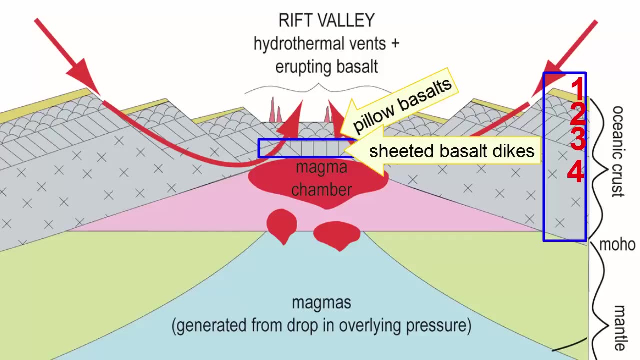 The magma that erupts on the seafloor cools quickly under high pressure cold water and forms structures that look similar to hardened toothpaste squirted out of a tube. They're called pillow basalts. The cracks in the crust that fed the magmas to the surface cool to form vertical walls. 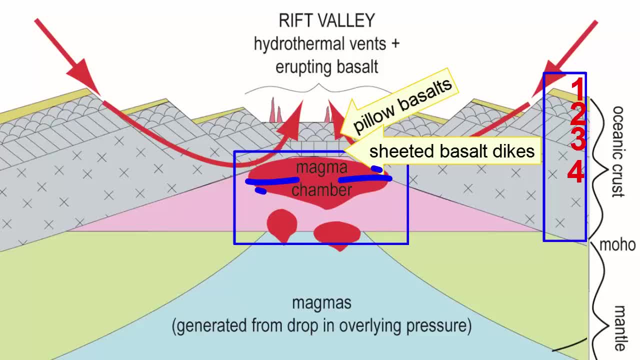 of basalt, called sheeted basalt dikes. The chambers that hold the magmas under these ridges will also spread. As their outer edges cool, they crystallize slowly to form a larger crystal rock with the same composition as basalt, but now called gabbro. 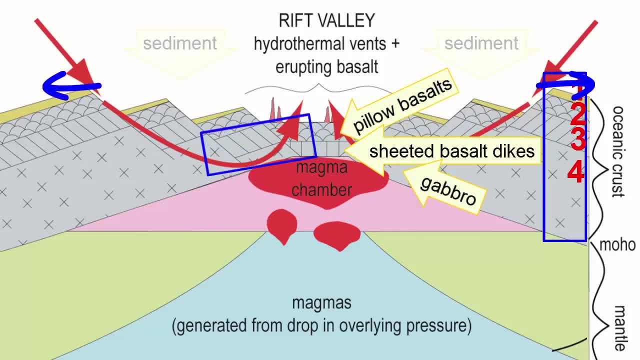 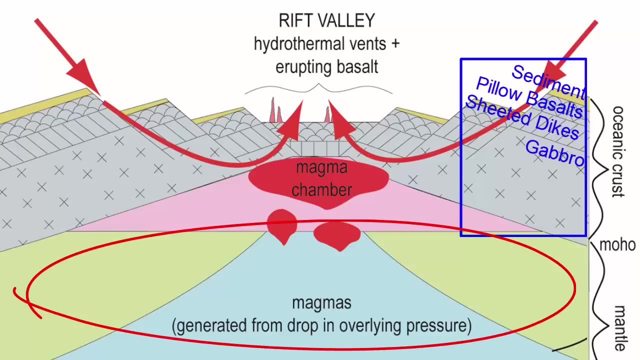 As this crust spreads apart to allow new crust to form between it, the ocean will deposit fine grains of dust, ash, shells and other debris. These are the four layers of ocean crust. Under the ocean crust is the mantle rock that melted to produce the magmas in the first. 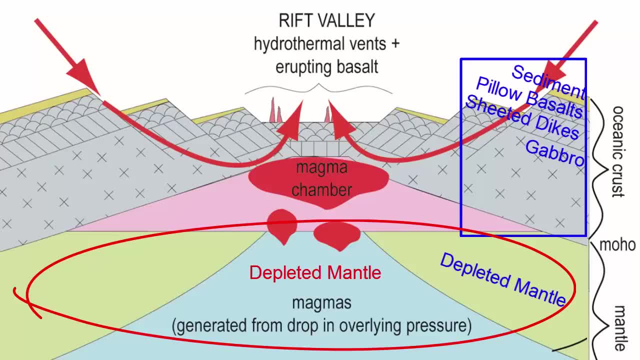 place. It is sometimes referred to as depleted mantle because it has had magmas produced from it, And it is attached to and under plates, the crust above it, making up the base of the ocean lithosphere. So ocean lithosphere everywhere in the world is basically made of this same sequence of 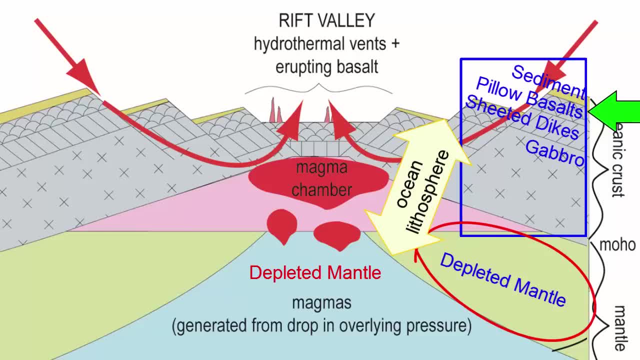 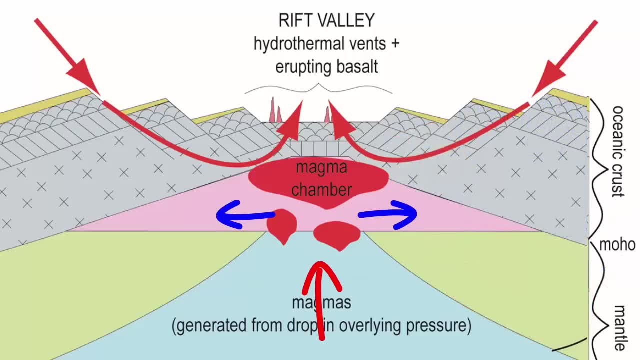 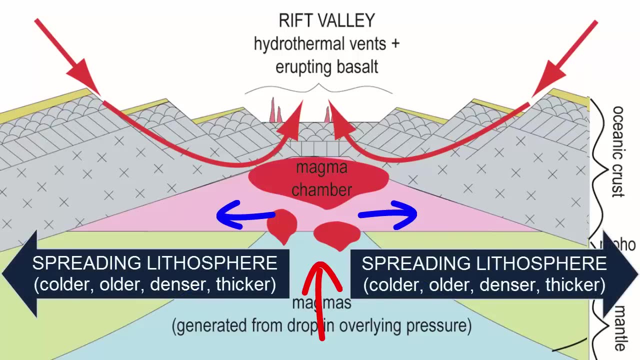 rock Sediment of varying thicknesses, above pillow basalt, above basalt dikes, above gabbro, above mantle rock. And what happens to this ocean lithosphere as it spreads? Not much. It grows gradually colder and older and denser and collects a thicker sequence of sediment. 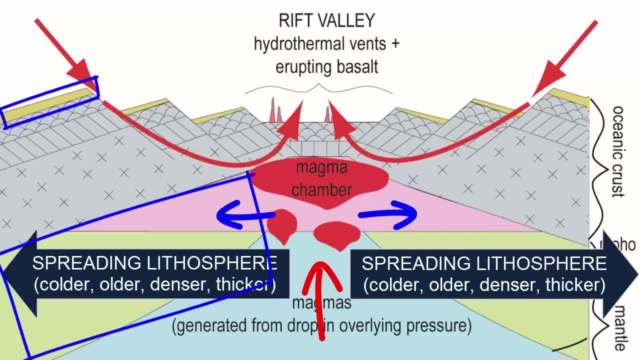 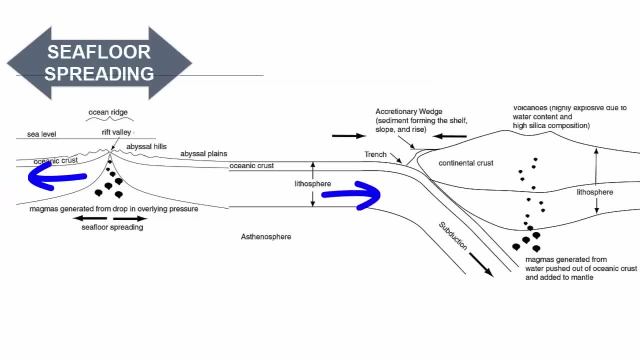 atop and a thicker section of mantle plating underneath it, thus thicker lithosphere, Until eventually it's so dense that it becomes denser than the rock underneath it. It detaches and sinks back into the mantle, possibly sinking or subducting as deep as the core. 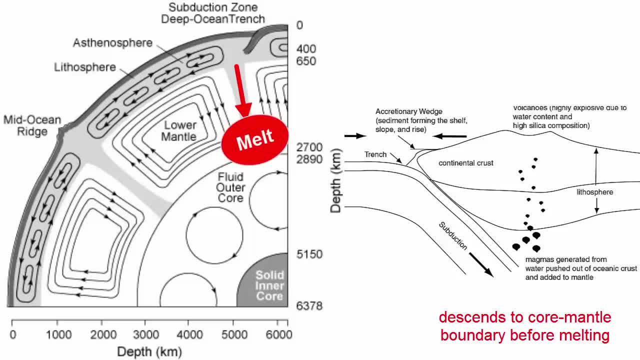 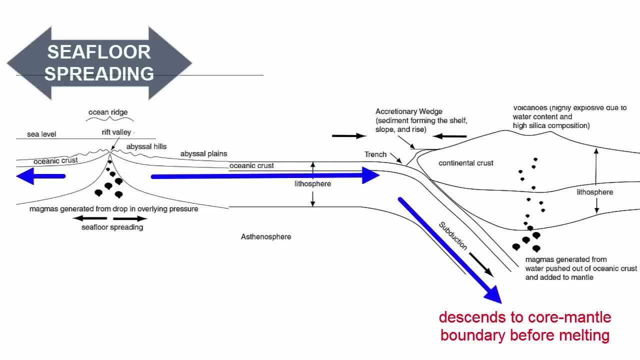 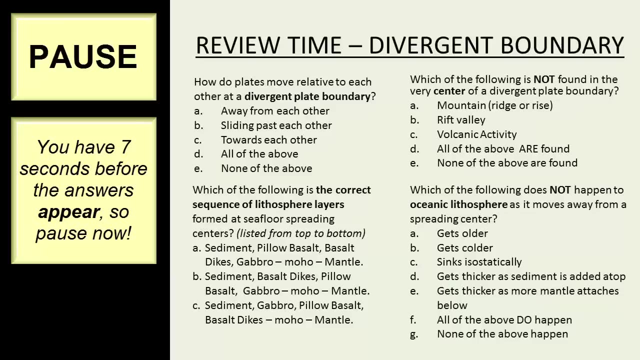 mantle boundary before finally melting and becoming reabsorbed back into the mantle Dense, cold lithosphere sinks down, pulling the distant seafloor spreading center further apart, driving together a recycling engine for mantle material. Pause now. Pause, now Pause. 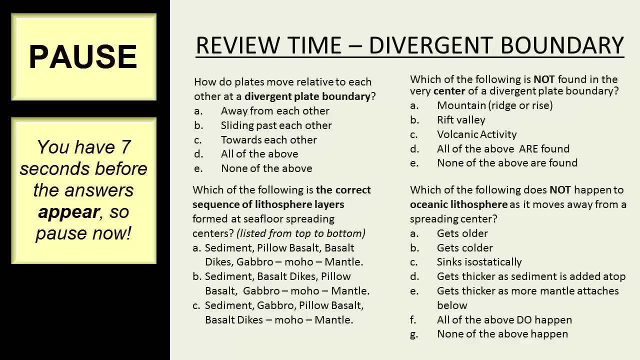 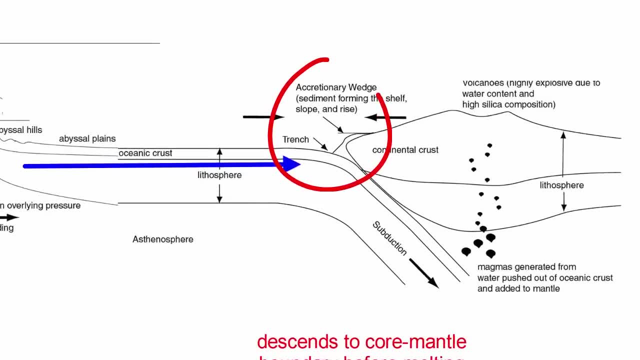 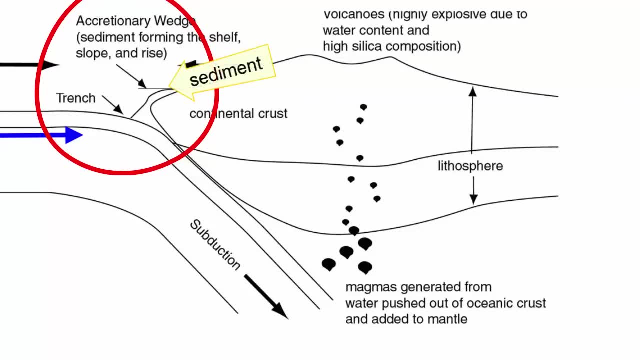 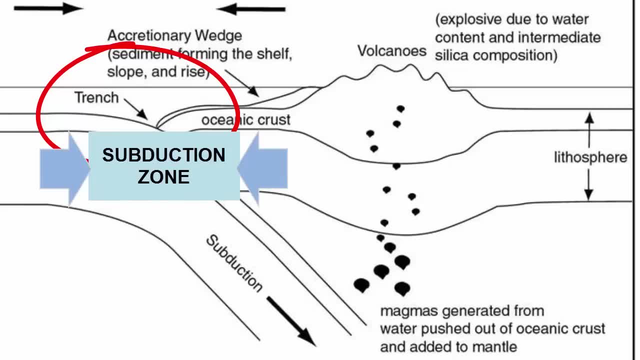 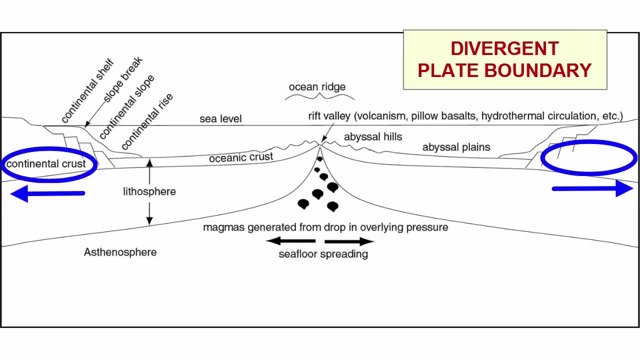 Let's look more closely at these subduction zones. Remember that at divergent plate boundaries the plates move apart. The old continental portions of these plates that were torn apart are also now spreading further and further apart. What happens at the outside of this spreading? where? 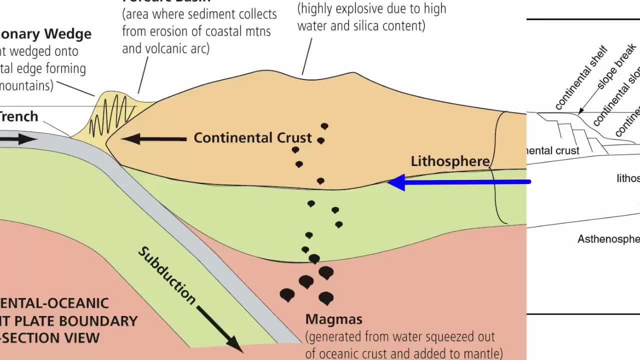 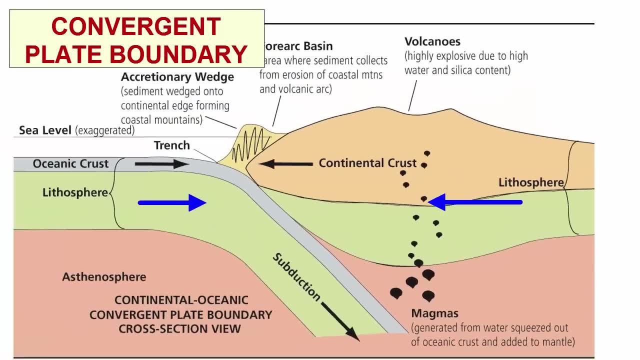 continents are shoved towards other plates, They will collide at boundaries referred to as convergent plate boundaries. If continents collide with ocean plates, the ocean plate being denser will be forced under the continents. If the ocean crust is cold and dense, it will sink to the core. 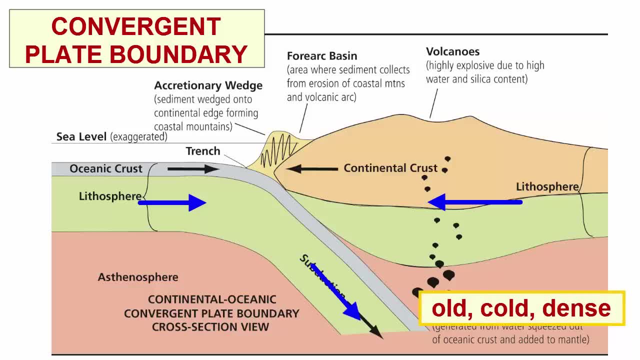 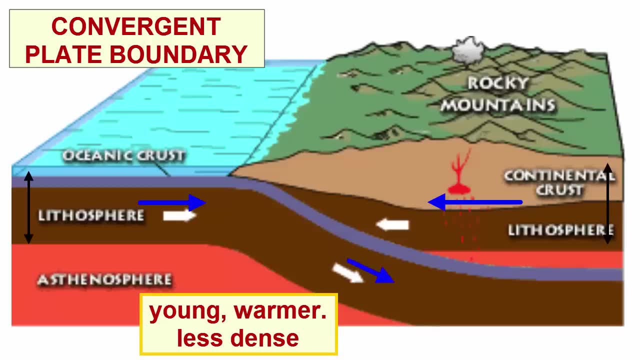 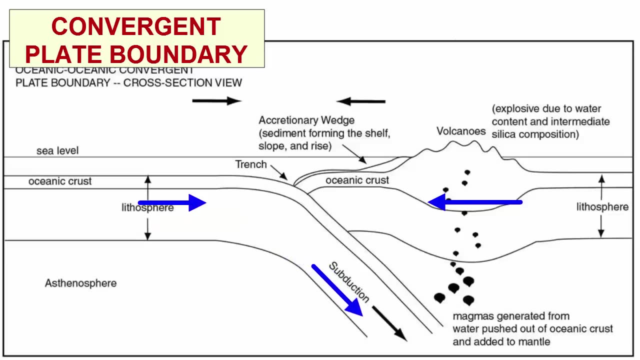 mantle boundary to be recycled, as already discussed. If the ocean crust is young and is not yet dense enough to sink, it will push under the continental plate and cause the continental crust above to be deformed. Convergent plate boundaries can also exist between two ocean plates, if one. 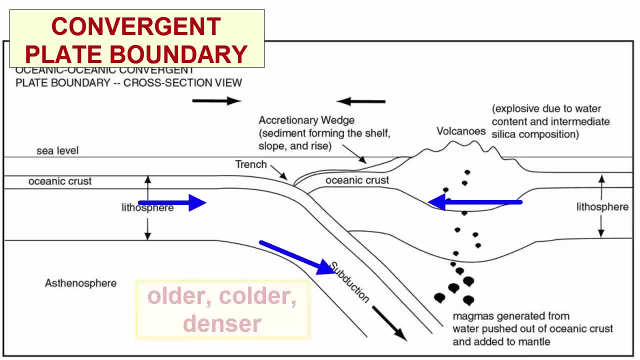 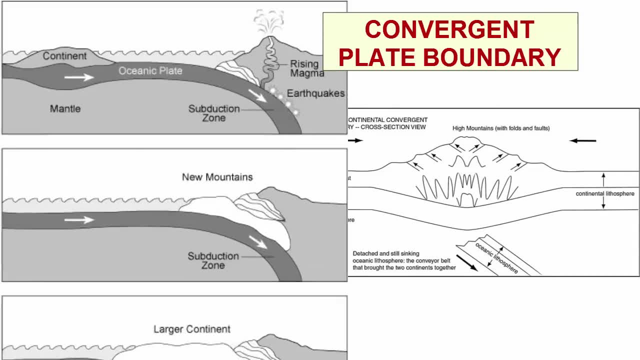 plate is much older than the other and convergence brings the two together. The older one subducts under the younger one. Convergent plate boundaries can also exist between two continents when the ocean that existed between them entirely subducts and the two collide and accrete together to form a larger continent. Convergent plate boundaries can also exist between two continents when the ocean that existed between them entirely subducts and the two collide and accrete together to form a larger continent. Convergent plate boundaries can also exist between two continents when the ocean that existed between them entirely subducts and the two collide and accrete together to form a larger continent. Convergent plate boundaries can also exist between two continents when the ocean that existed between them entirely subducts and the two collide and accrete together to form a larger continent. Convergent plate boundaries can also exist between two continents when the ocean that existed between them entirely subducts and the two collide and accrete together to form a larger continent. 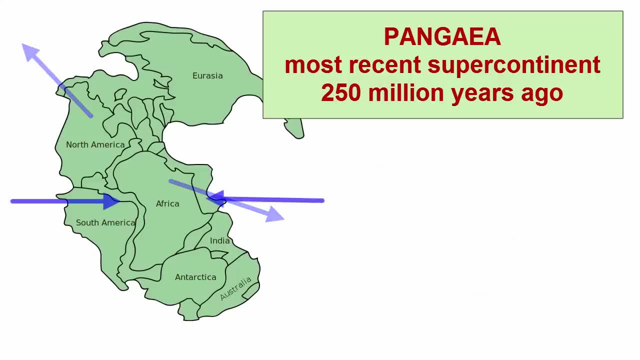 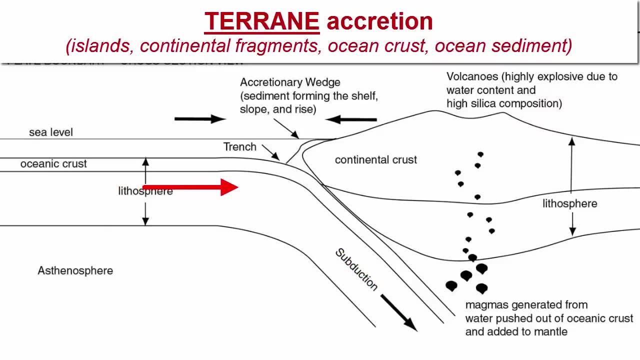 Just as divergence is the method for breaking up continents, convergence is the method for conjoining them. In fact, even as ocean floor still exists and subducts alongside a continent, accretion and continental growth is happening. Islands, continental fragments, sediment and the crust that carries them can get 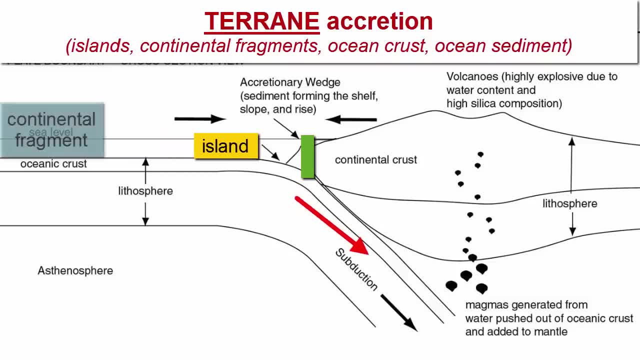 scraped off and accreted to the edges of the continent. We call these accreted fragments terrains, and they are the basic building blocks of all continents: terrains, and they are the basic building blocks of all continents. continental material are the volcanic eruptions that happen alongside the subduction. why, when? 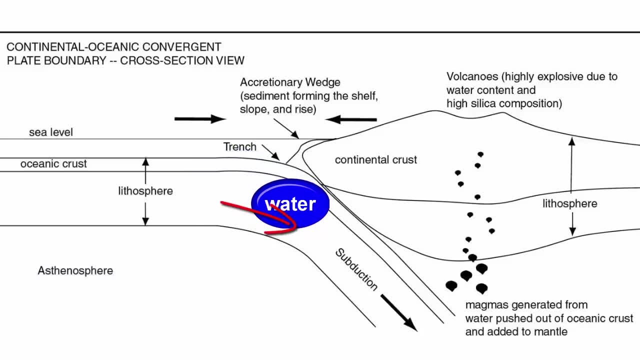 ocean crust subducts, it carries with it a large amount of water that has soaked into the sediment over millions of years. that water is squeezed out by the high pressure at depth in a subduction zone. because water is less dense than anything else, it rises upwards into the overlying asthenosphere. 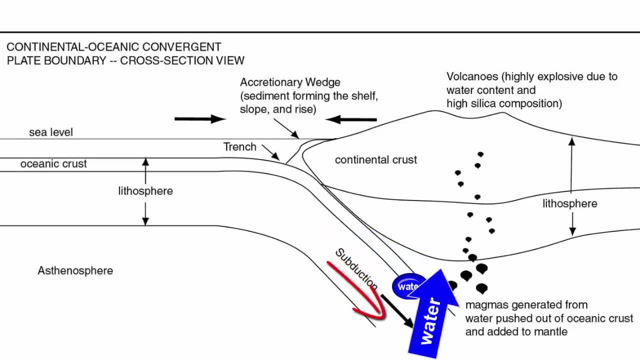 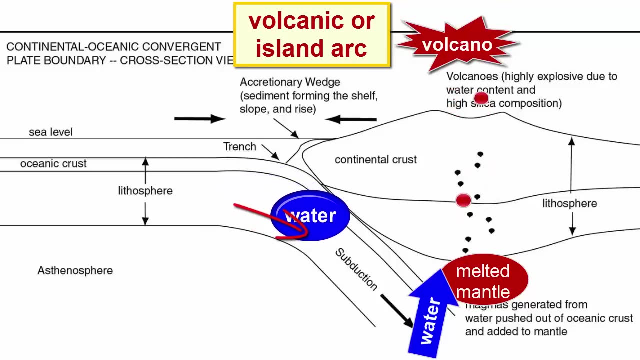 water reduces the melting point of the asthenosphere, causing it to melt. that molten magma is now less dense, and so it too rises with the water to the surface, where it erupts in a chain of active volcanoes known as a volcanic arc or island arc subduction zone volcanoes. 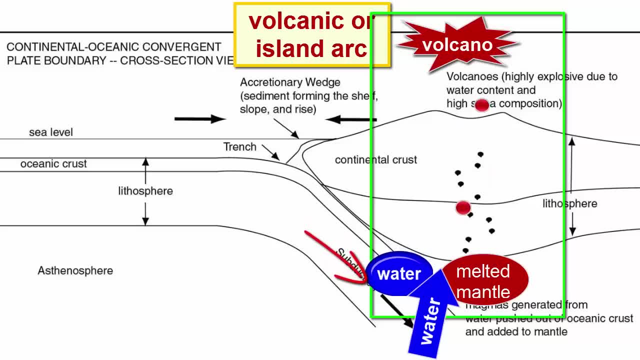 always happen above the subduction zone on the plate. that does not subduct and produces some of the most hazardous volcanoes in the world. why, among other things, all that water can produce high amounts of pressure underground. does continental crust ever subduct? no, why not? it's the least dense material on the planet. 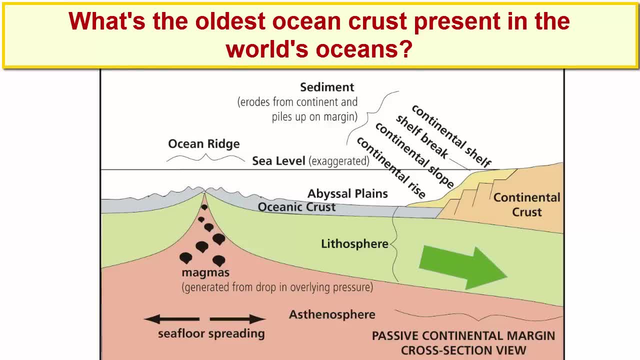 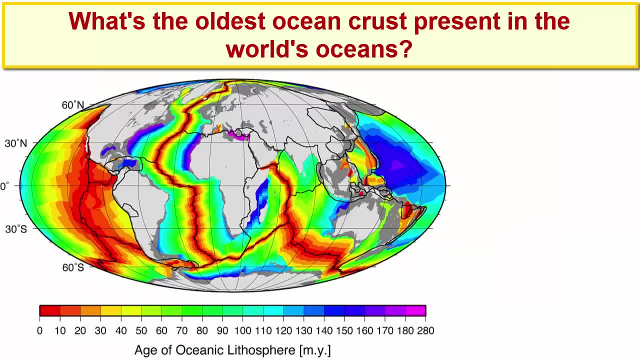 how old does ocean lithosphere need to be before it detaches and subducts all on its own? all we can find to answer that question is the age of the oldest ocean rock currently residing in the oceans, and that's 200 million year old rock subducting under the marianas trench in the pacific. 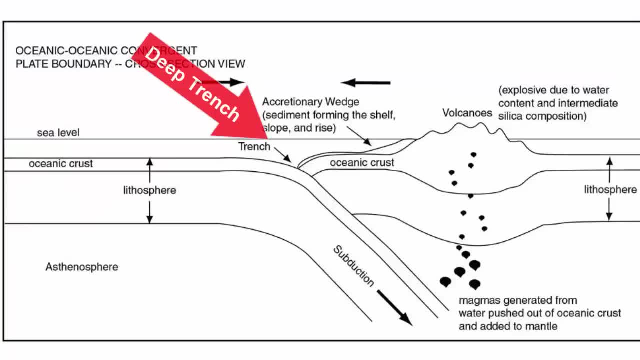 why is the marianas trench the deepest part of the planet? because it's a converging plate boundary where two of the ocean's most dense rocks are subducted under the marianas trench in the pacific. why is the marianas trench the deepest part of the planet? because it's a converging plate boundary where two 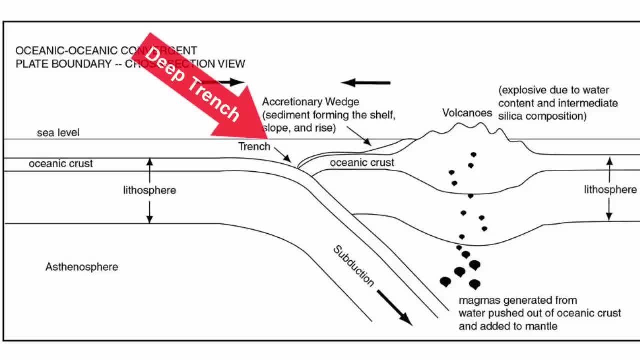 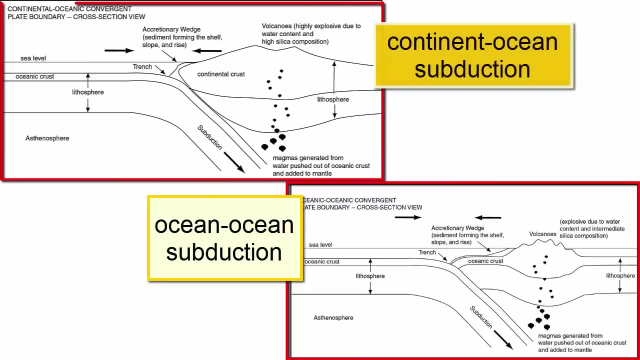 ocean plates are colliding. that means that both plates are already riding low isostatically. now combine that with one subducting under the other and no nearby continents to fill the trench with sediment, and there you have an answer. do ocean ocean subduction zones produce the same types of features as continental ocean subduction zones? 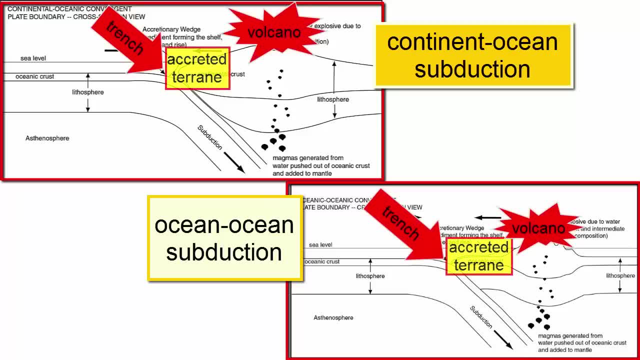 trenches, volcanoes, accreted terrain, material that forms coastal mountain ranges. yes, the only difference is that the volcanoes erupt through thinner oceanic lithosphere. yes, the only difference is that the volcanoes erupt through thinner oceanic lithosphere, and that makes them slightly less dangerous than the magmas that rise through thicker continental. 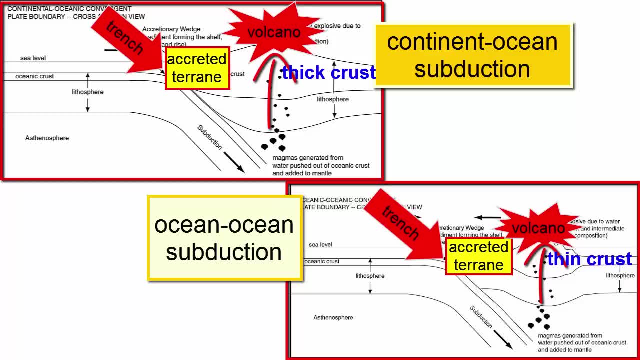 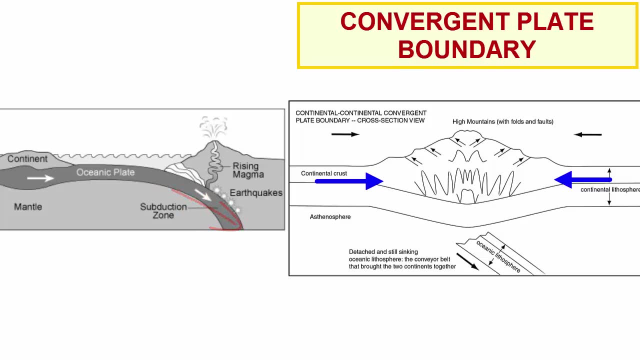 lithosphere. why? the thicker the lithosphere, the more likely the gas content will increase in the magmas, and this gas leads to higher pressures and more explosive volcanoes. let's look again at what happens when two continental plates collide. subduction brings the two together, but then, after they collide, the subducting 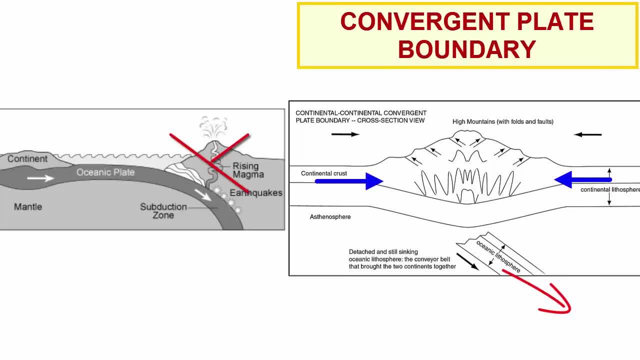 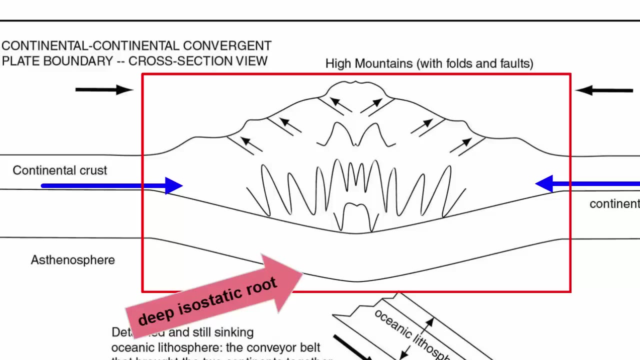 plate completely detaches and sinks into the mantle, volcanism stops, the trench disappears and the largest mountains found on the planet form, as terrain accretion mashes the two continents up into a folded, faulted mountain system that rises high above the surface and has a deep isostatic root beneath. 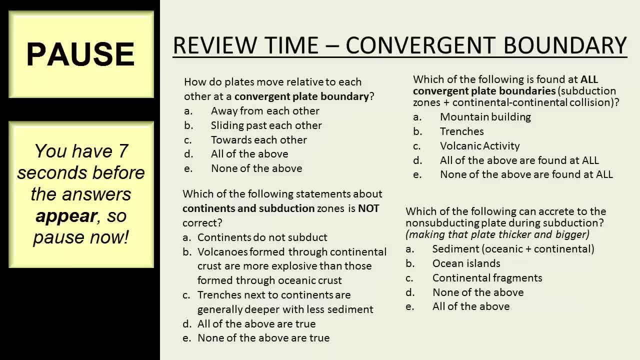 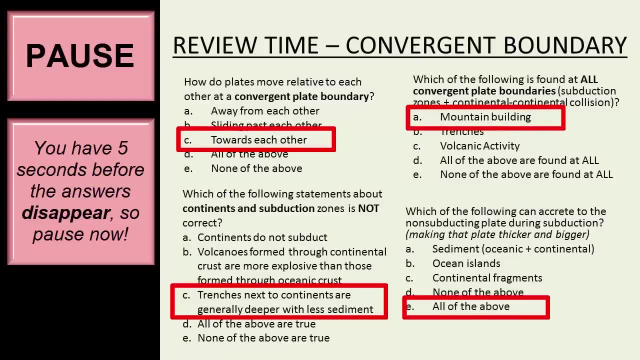 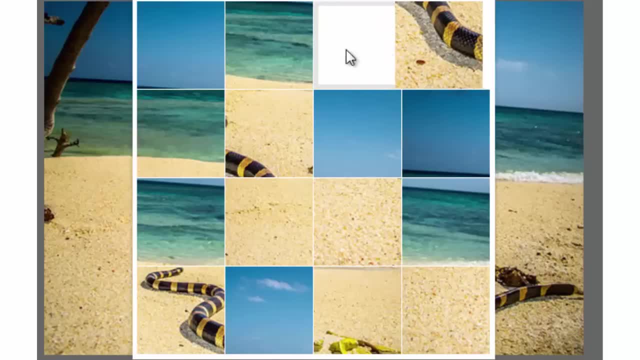 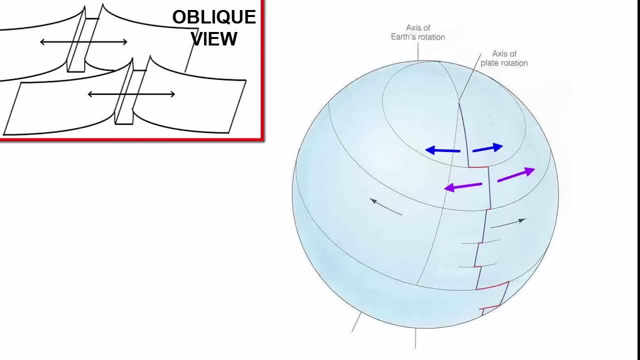 pause. now that leaves one remaining plate boundary to discuss: transform. transform where plates slide past each other. there's no way to have plate motion moving apart and together without having some edges slide past each other. it's really easy to see how transform plates form when we look again at divergent plate boundaries and remember that the 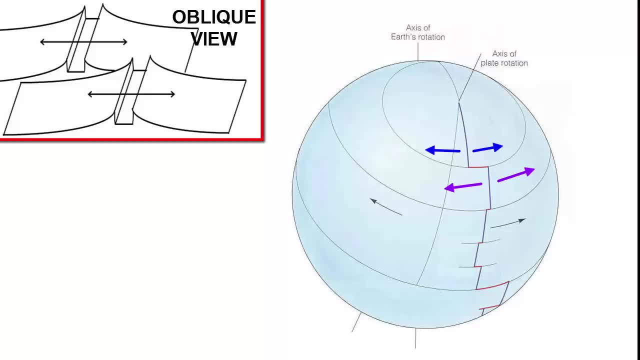 tearing apart of the lithosphere has to accommodate a spherical surface, like seams on a baseball. it's hard to sew together or pull apart two pieces of fabric on a spherical surface without buckling or tearing to accommodate divergent motion along ridges that run along a spherical 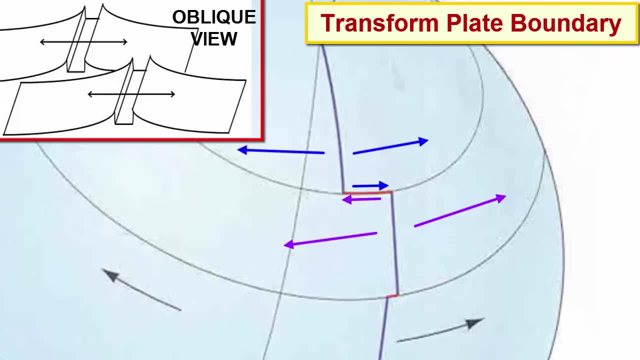 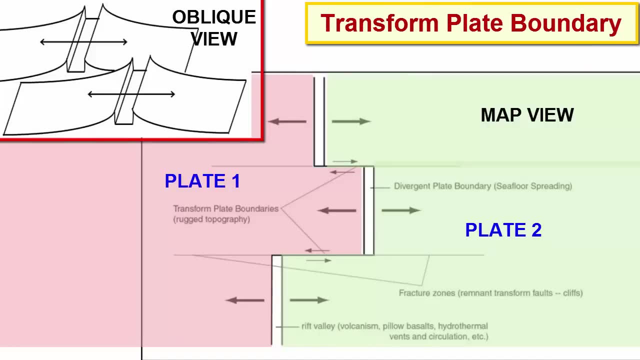 surface. the ridges break into sections and each section is offset from the next one by a transform boundary. as this image shows, there are two plates, but in these zones the boundaries are divergent. in these zones, the boundaries are transformed. let's test our understanding with a few questions. 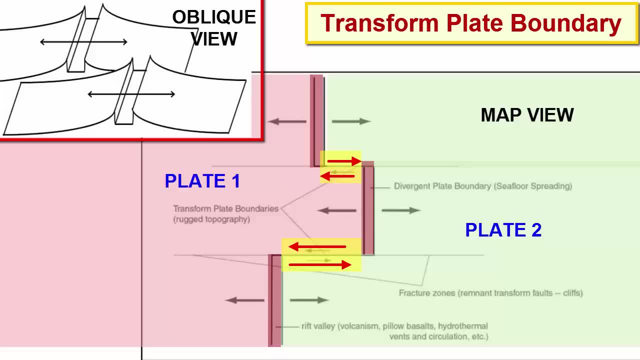 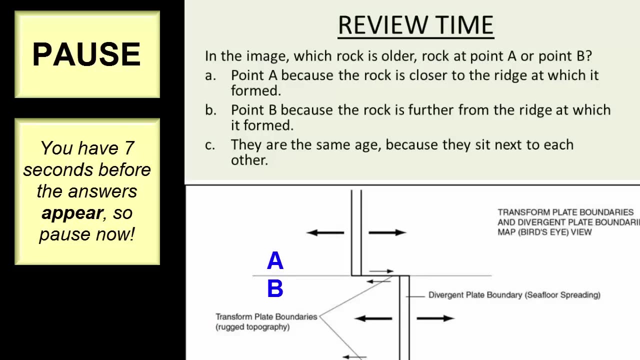 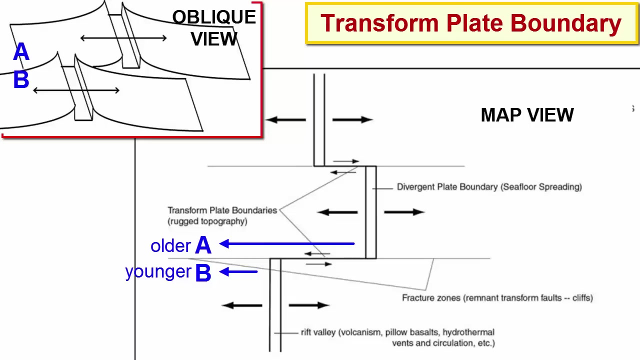 where is the youngest rock in this image? let's put a y there. where is the oldest rock? let's put an o there. how do points a and b compare? pause now. rocks at point a and b formed at different locations, but are now found alongside each other. 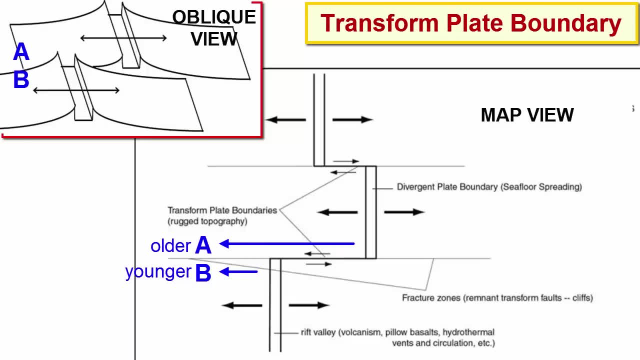 so they will look very different. they will have different thicknesses of sediment. the younger one will be higher in elevation. there will be a cliff between them, and that cliff marks a line that runs outward from the active, transform faults and creates a spectacular scar. We call this old scar a fracture zone.